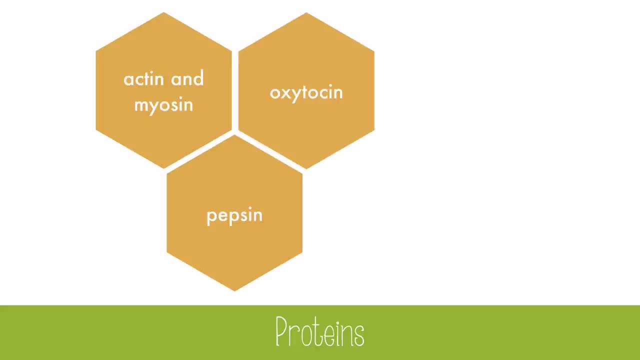 proteins are also enzymes and many enzymes end in ace, like catalase, which rapidly turns hydrogen peroxide into water and oxygen, or lactase, which breaks down lactose in milk. If you are lactose intolerant, you don't make enough of the enzyme lactase. 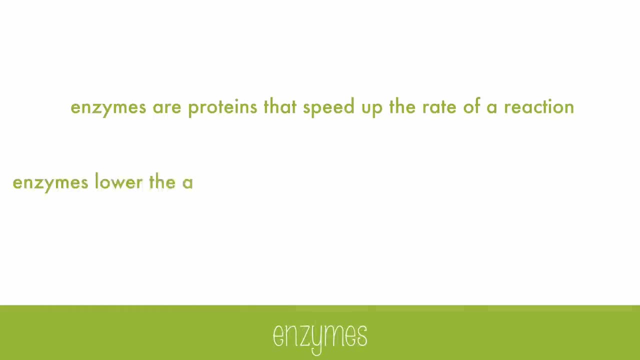 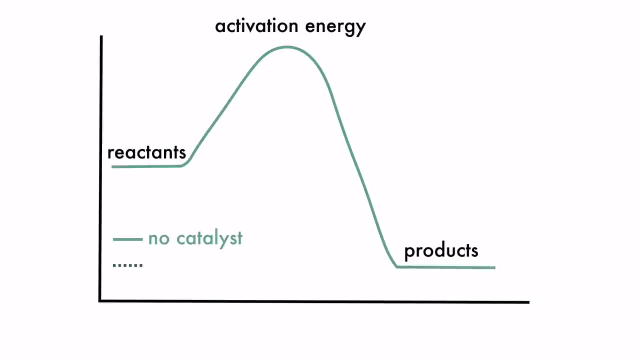 Enzymes are proteins that speed up the rate of reaction. They work by lowering activation energy required for the reaction to begin. Here's what that looks like. A normal reaction has a certain amount of starting energy, or activation energy, that's required before the reaction can truly begin and create product. 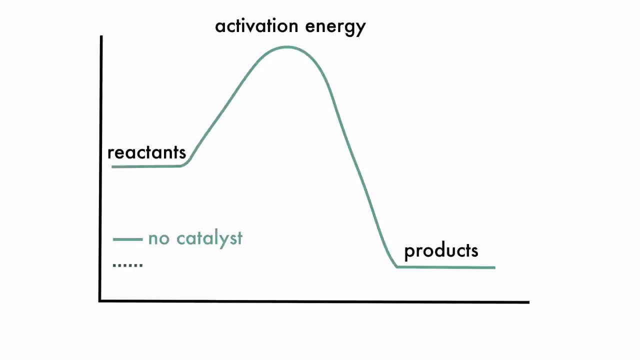 So let's confirm, because with no catalyst, like an enzyme, the reaction might be relatively slow, But with a catalyst, the activation energy is decreased and the reaction can occur faster. It's like being able to drive your car through a tunnel instead of up and over a mountain. 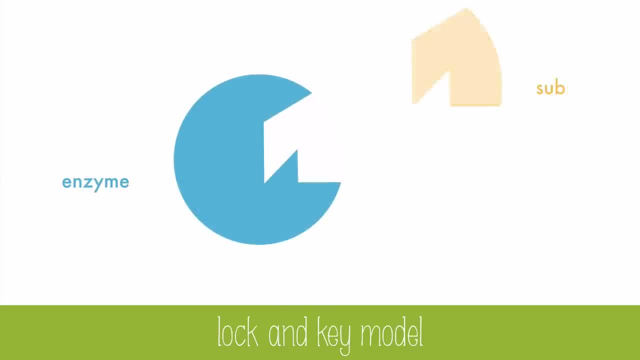 it's much faster. Enzymes work only on one specific substdle. The enzyme and substrate fit together like a lock and key. In this example, the substrate is broken down into two products, But some will put things together. Proteins have many different functions. 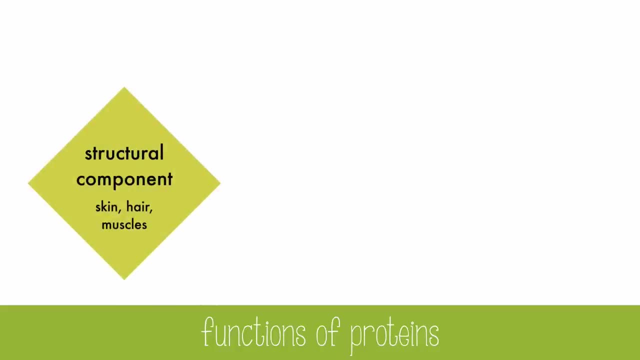 There are structural components of which much of the body is made, including skin, hair and muscles. Proteins are also chemical messengers. like hormones, They assist in defending our bodies against disease in the form of antibodies, And many proteins are enzymes, like catalase and lactase. 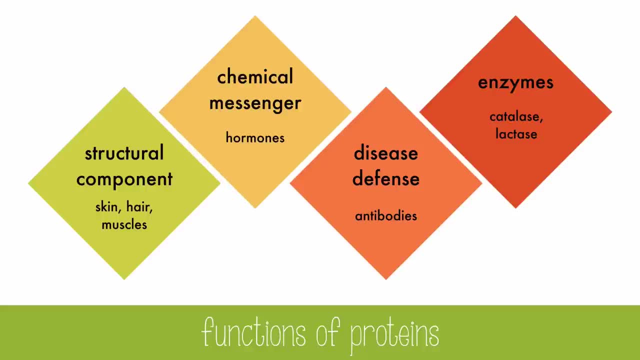 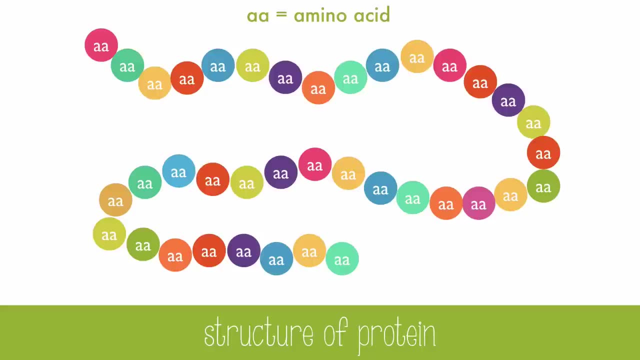 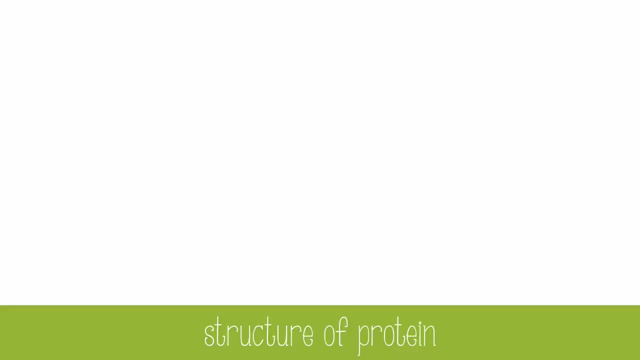 speeding up reactions and working over and, over and over again. Proteins are made of long chains of amino acids and they're linked together by peptide bonds. These long chains of amino acids, also known as polypeptides, will coil up and form a functional protein. 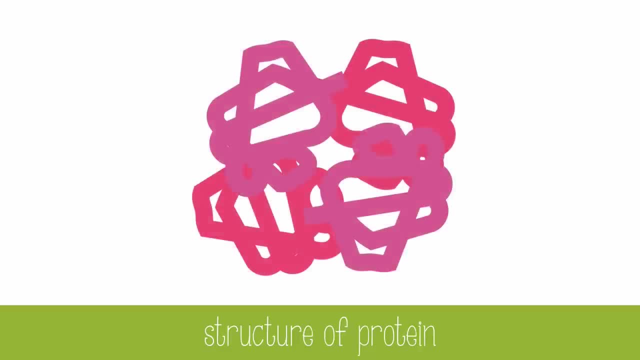 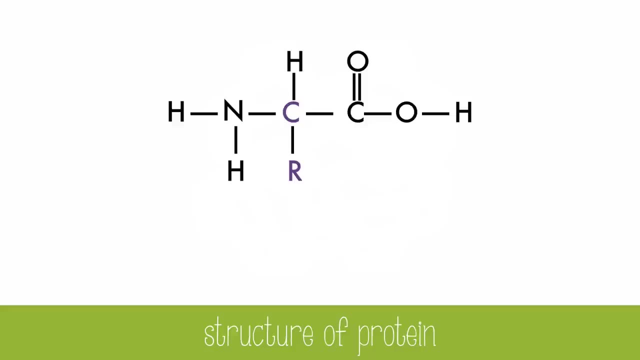 The protein will not work until it's folded up correctly. Proteins are different from one another because they are made of different combinations of amino acids. Amino acids have a basic structure of a carbon, a hydrogen, an amino group, a carbon, a carbon.